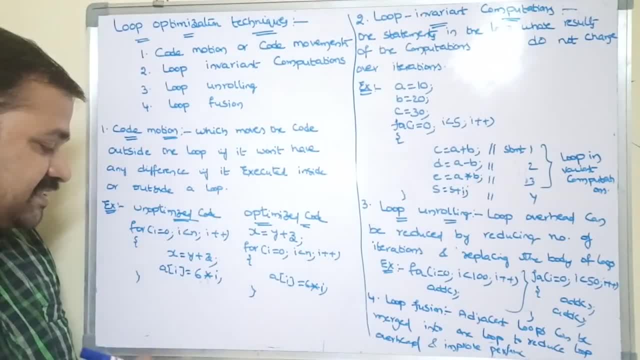 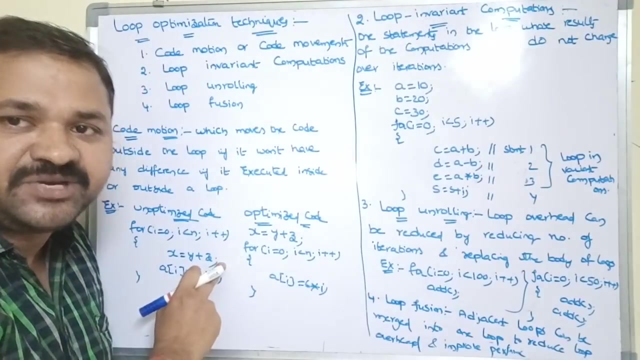 be executed 10 times, so throughout the 10 iterations the value of x should be constant. only the value of x won't changes. so in this type of situation we can move the statement outside the loop so that the statement is executed only once, whereas if it resides in the loop then it is. 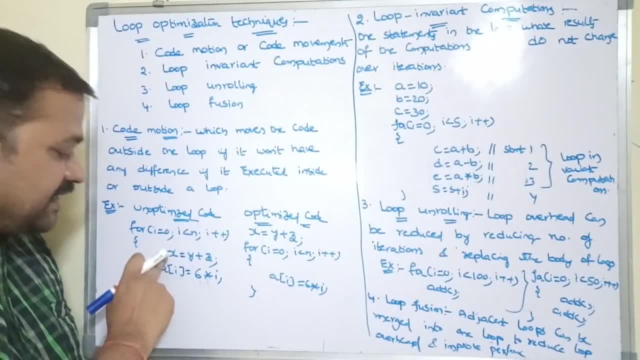 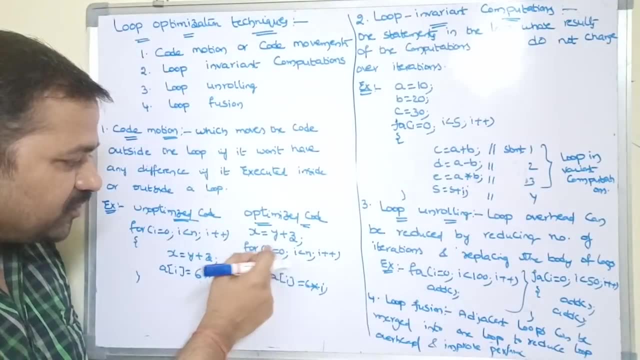 executed then depends upon the number of iterations. here the statement is not depending on this for loop, so we can move the statement outside the loop. so the optimized code is: move the statement above the far loop. so x is equal to y plus z. why? because if we move the statement above the far 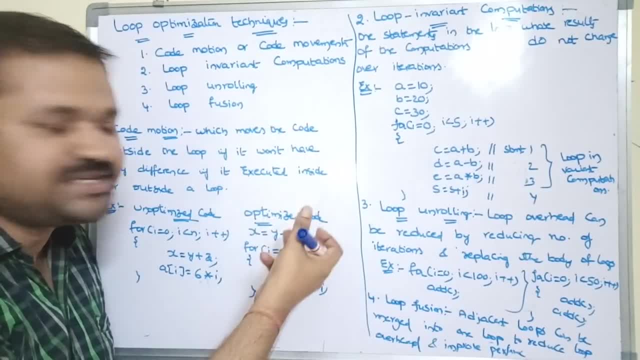 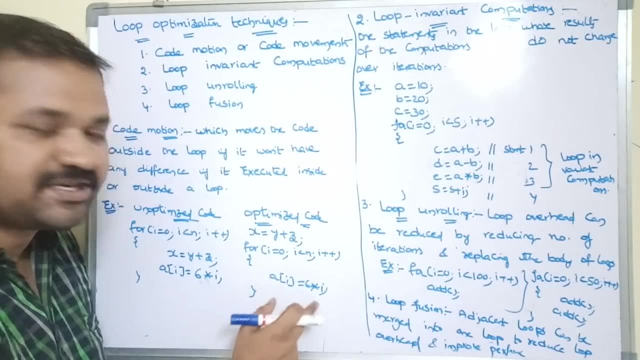 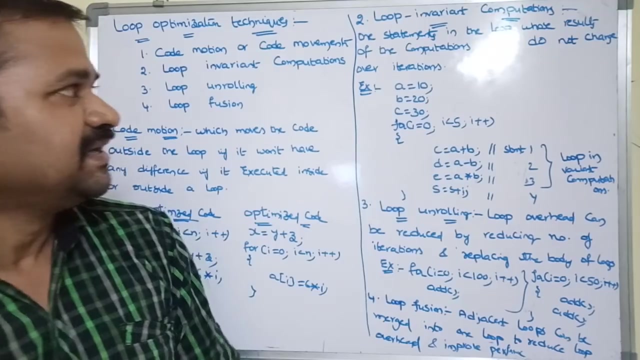 loop, then the result of x won't changes if it executed inside or outside the loop. so for, i is equal to zero, i less than yet, i plus less. so what is the body here? a is equal to 6 into i. now let's see the next approach. the next approach is loop invariant computations. let's see what is the. 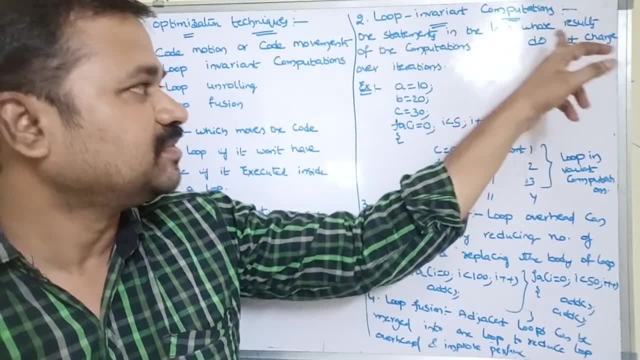 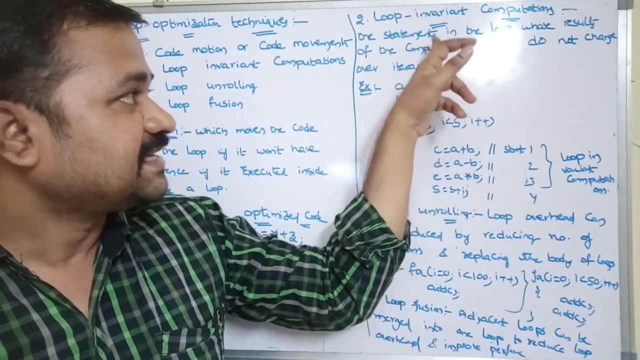 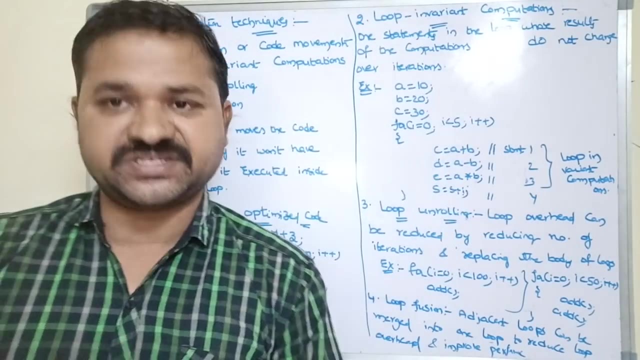 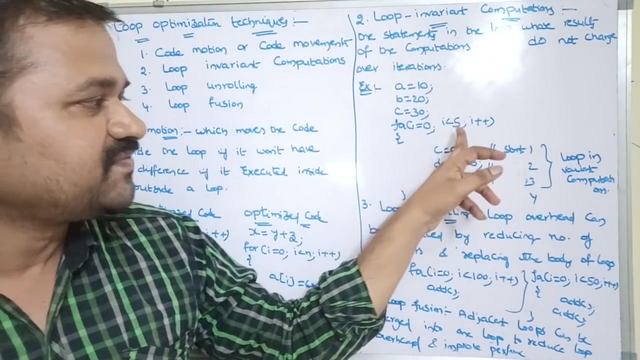 loop, invariant computations. invariant computation: the statements in the loop whose results of the computations do not change over the iterations. the statements in the loop whose results of the computations do not changes over the iterations. so now let's see an example. let a value is 10, B value is 20, C value is 30, so for I is equal to. 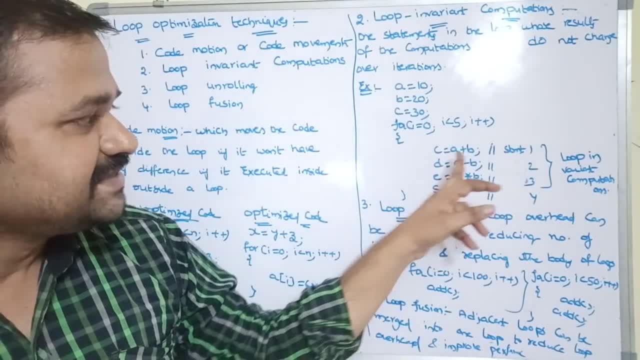 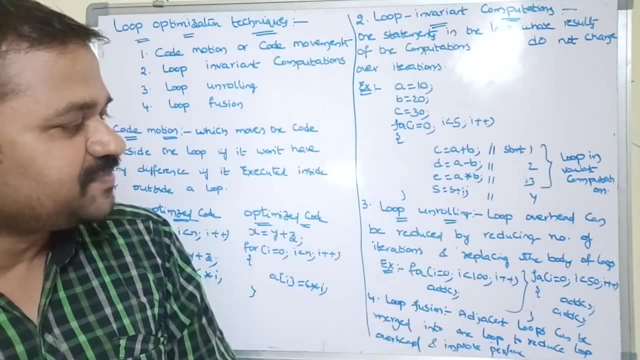 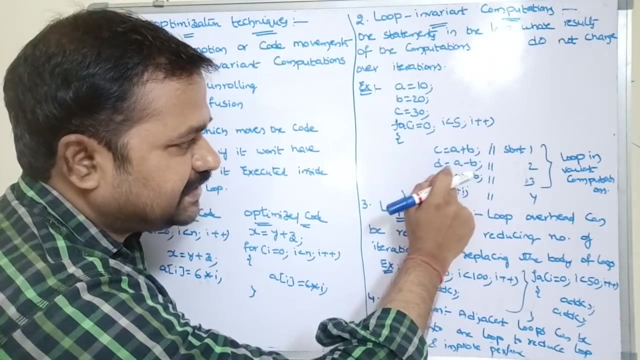 0, I less than 5, I plus plus. so C is equal to a plus B. D is equal to a minus B. a is equal to a star B. yes is equal to s plus I. if we observe the first two, three statements, C is equal to a plus B. D is equal to a minus B is equal to a. 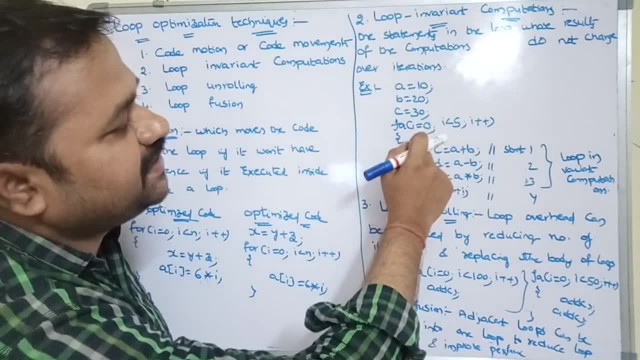 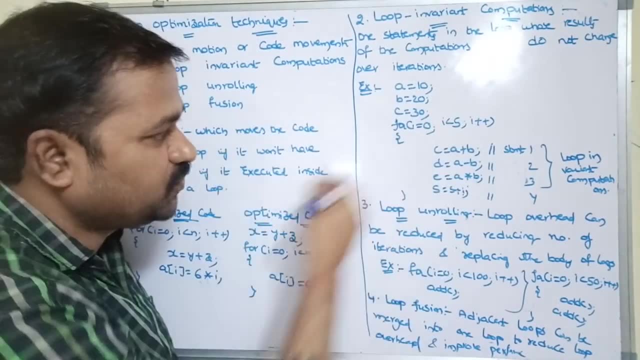 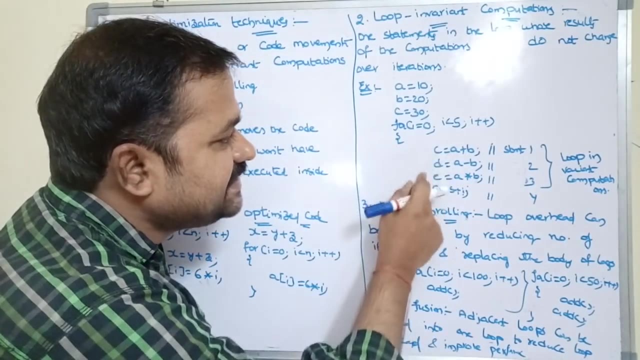 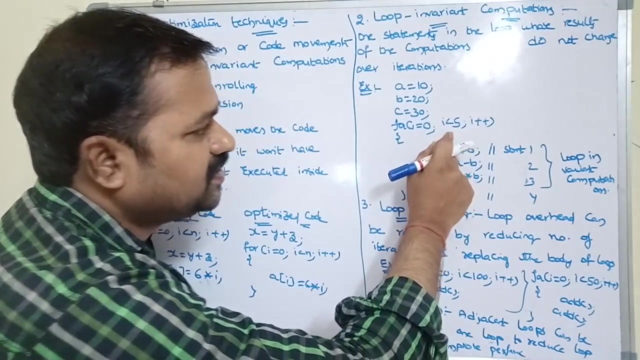 star B. here a B values are assigned above the for loop. so that means here a B values are not depending on the for loop. so these computations are known as the loop invariant computations. so we can eliminate this, these three statements here. why? because the result of C, D and E won't depends upon this for loop. because ABC are some constants. 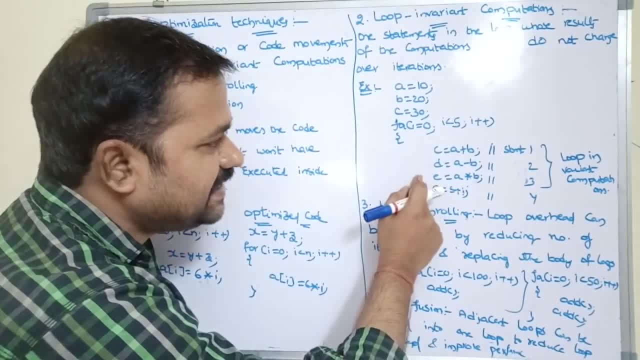 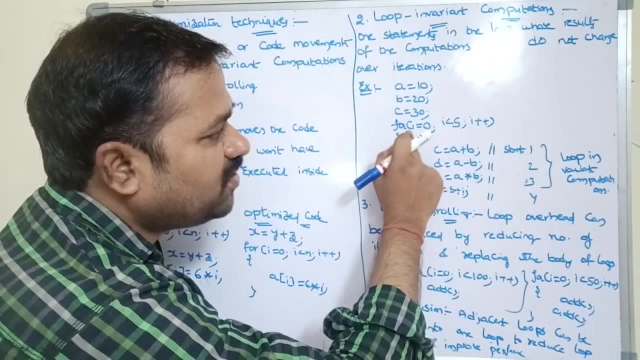 which are defined above the for loop. so we can place these statements above the for loop. whereas if you take the next one, yes is equal to s plus I. this statement is depending on this for loop, because here we have I. I depends upon the for loop, so this for loop should contain only this. 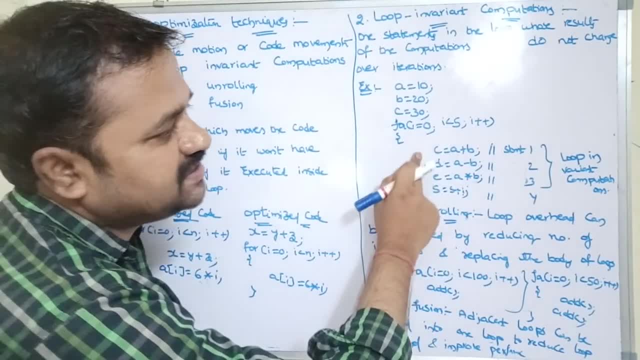 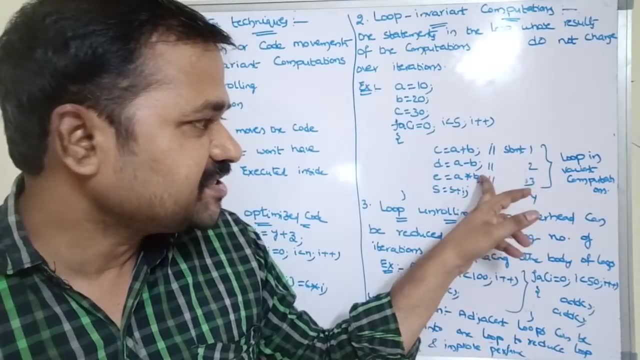 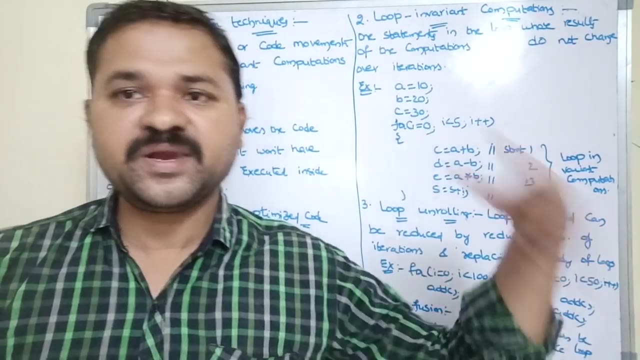 statement. we can eliminate these three statements. so these are nothing but loop invariant computations. so that means the name itself specifies the meaning. these computations are not depending upon the corresponding for loop. loop invariant computations. so computations are not depending upon the for loop. so we can eliminate these three statements and we can keep these three statements above the for. 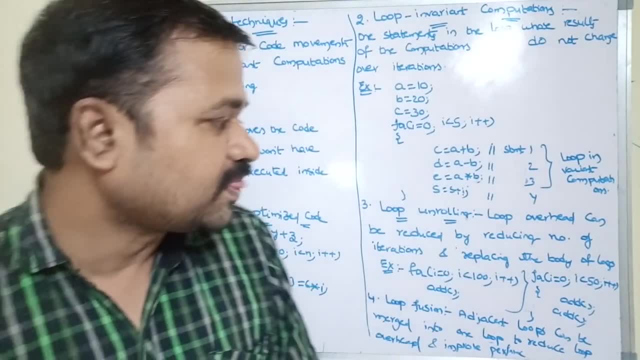 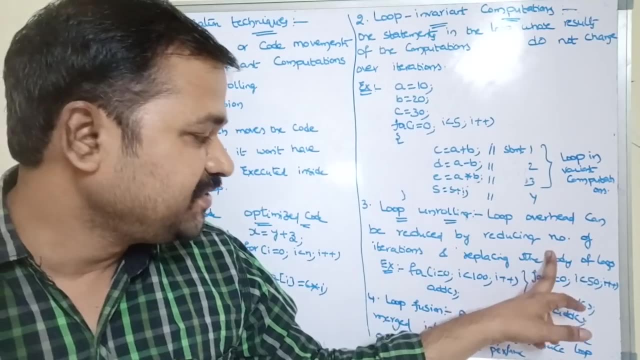 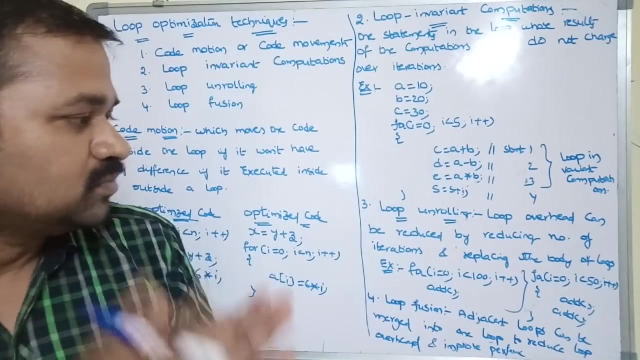 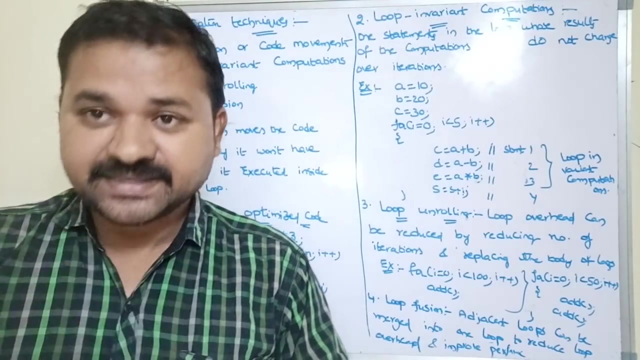 loop and the next one is loop unrolling. let's see what is loop unrolling. loop overhead can be reduced by reducing number of iterations and replacing the body of the for loop. so, in order to reduce the loop overhead, what we can do is we can reduce the number of iterations. 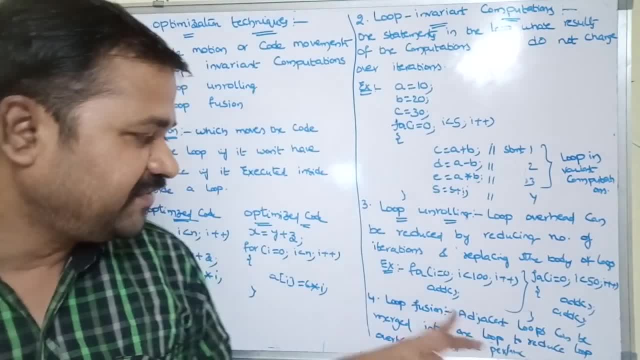 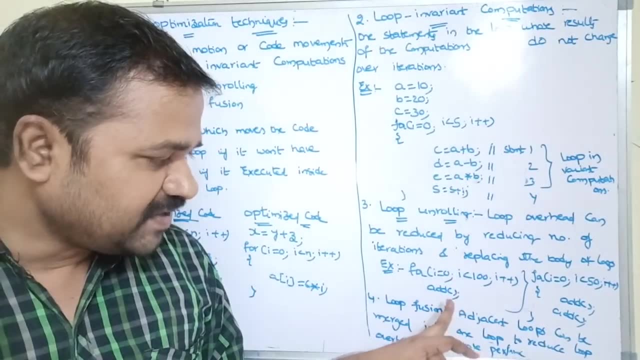 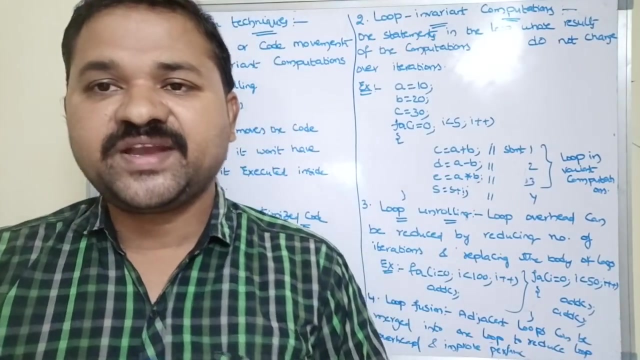 by placing more number of statements in the for loop. if you take an example: yes, for is equal to zero, I less than hundred, I less plus add function call. so what will happen? no, add function is called for 100 times, so too many times. we are calling the function. so whenever a function is called, then the control has. 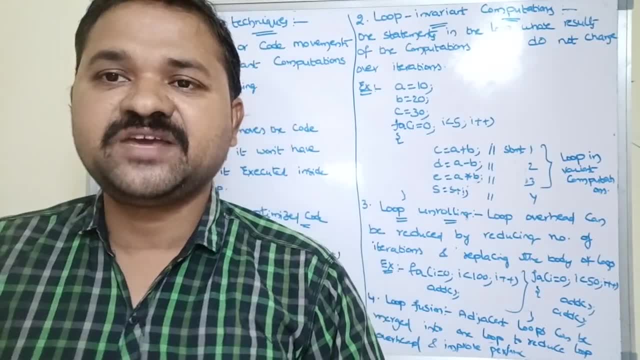 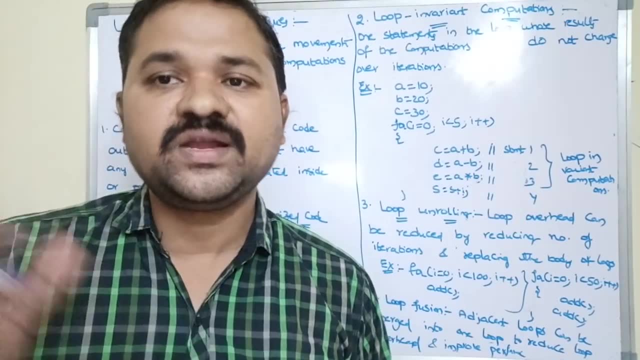 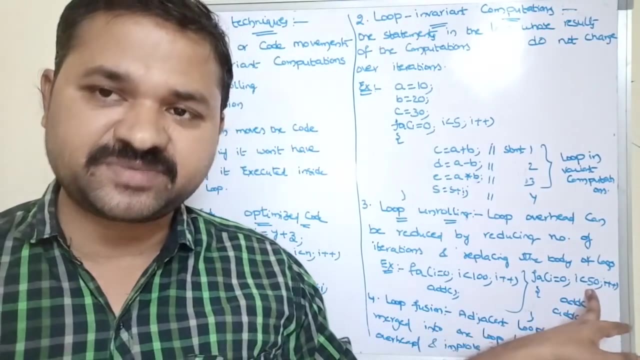 to goes to the function definition, and the function definition has to be executed. and once the function definition was successfully executed, once again control comes to the calling function. So there are too many activities while calling the function. So we can overcome this problem by repeating the for loop only 50 times. 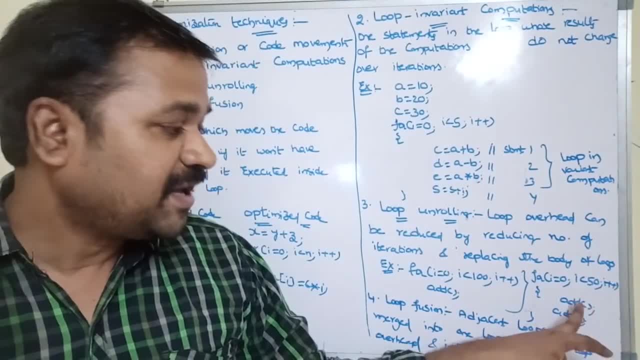 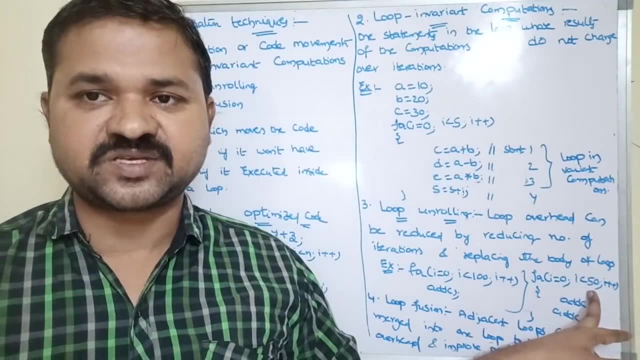 So for i is equal to 0, i less than 50, i plus less. But we are calling add function 2 times. So how many times we are repeating the for loop 50 times? So 50 into how many times we are calling the function 2 times. 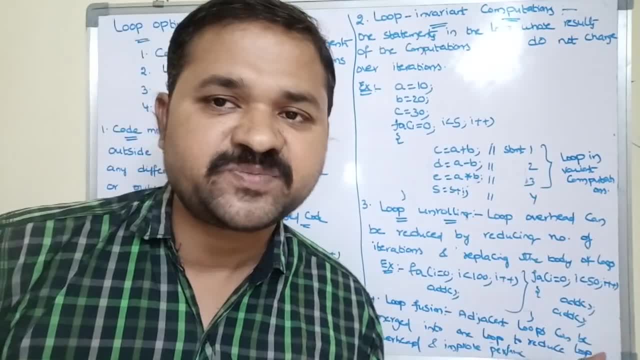 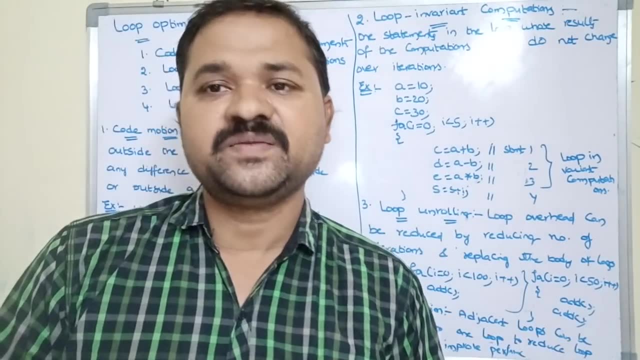 So 50 into 2 is nothing but 100.. So 100 times the corresponding function will be executed. So instead of calling the function 100 times, we are calling the function only 50 times only. We are repeating the for loop only 50 times only. 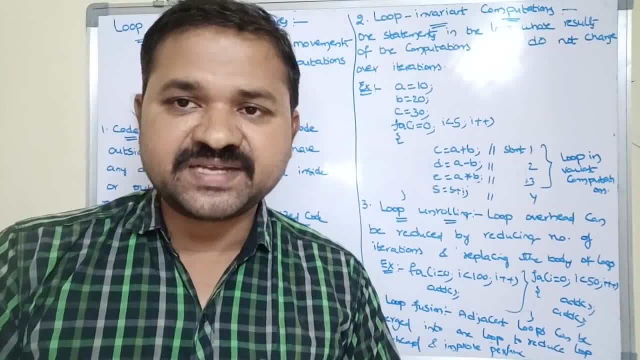 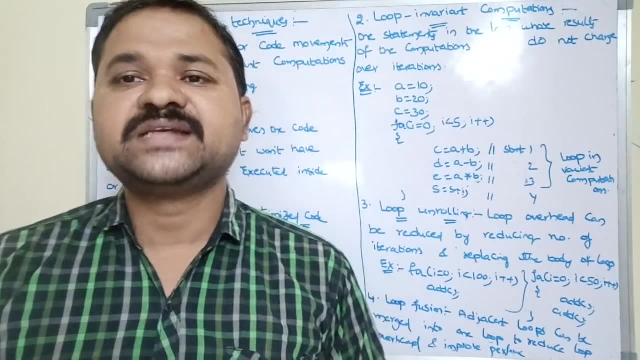 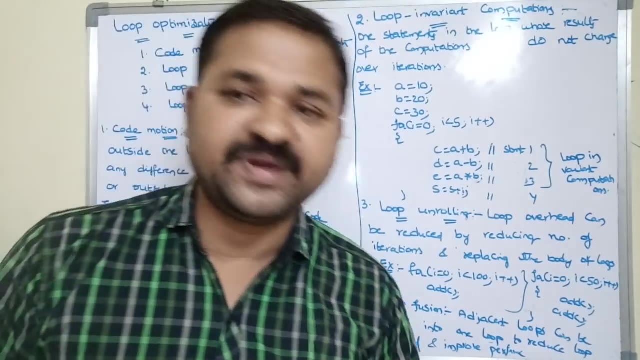 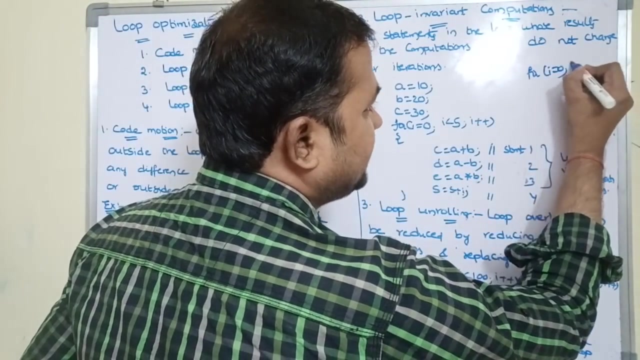 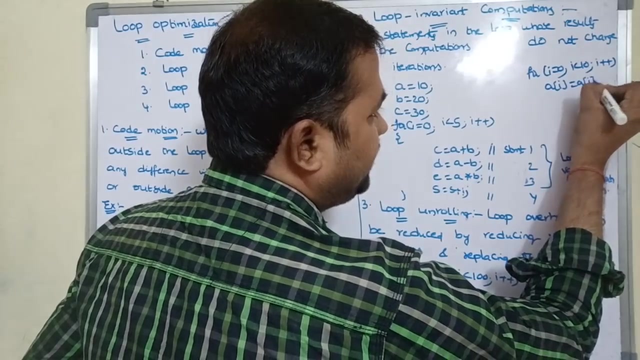 And the last one is loop fusion. Loop fusion is nothing but fusion, means merging. Merging of the several loops into a single loop is nothing but loop merging. So this will reduce the loop overhead As well as improve the performance. If you take an example as so for i is equal to 0, i less than 10, i plus less, a of i is equal to a of i into a of i plus 10.. 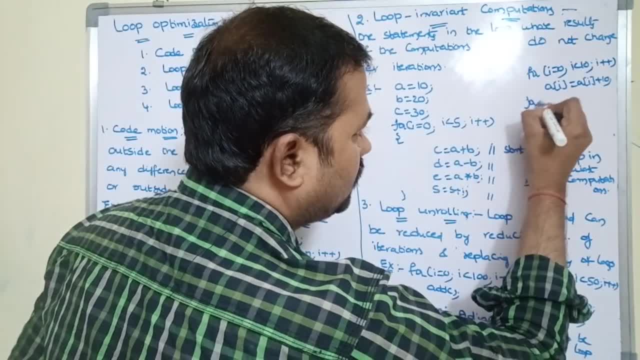 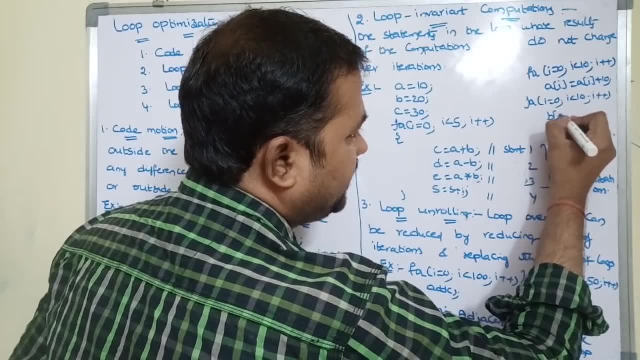 So this is nothing but one for loop. Second for loop: for i is equal to 0, i less than 10, i plus less b of i is equal to b of i plus 10.. So here we have two for loops. 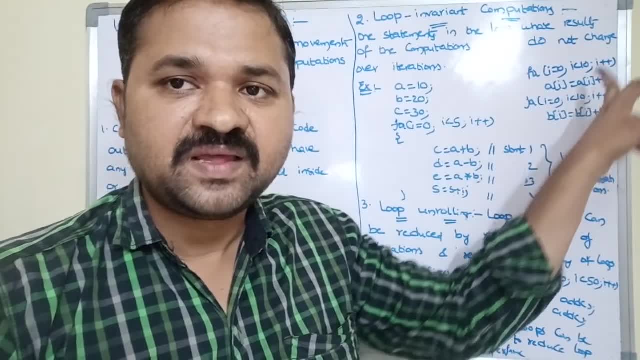 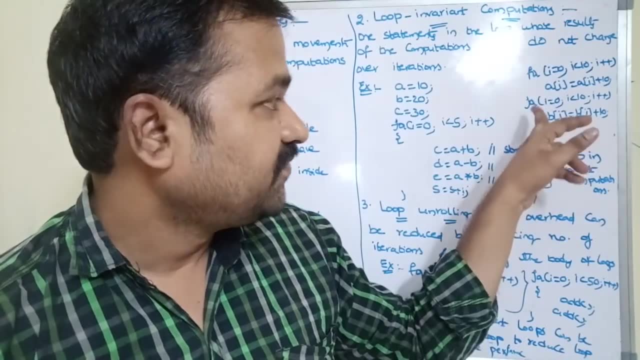 Initialization is same as well as condition is same as well as incrementation is same. For the first for loop, the body is a of i is equal to a of i plus 10.. For the second for loop, the body is b of i is equal to b of i plus 10.. 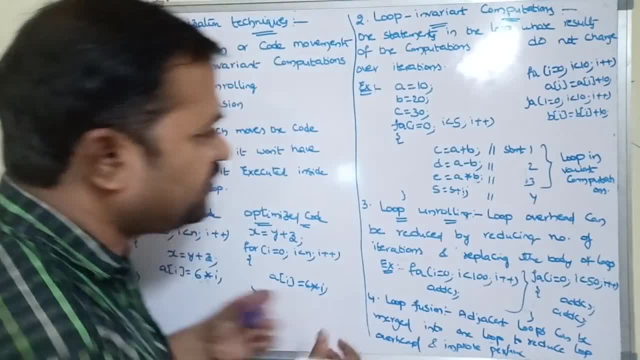 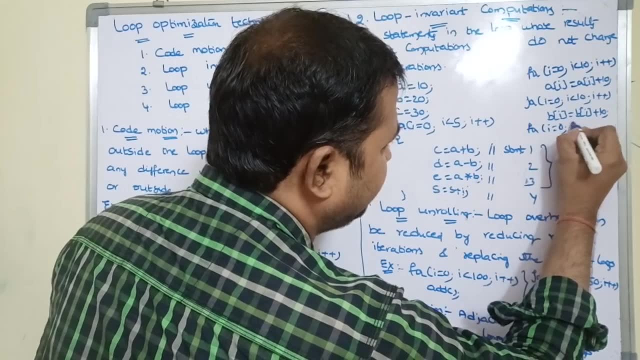 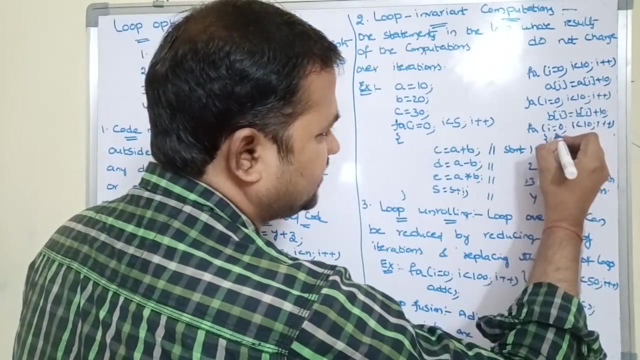 Now we can merge these two for loops into one for loop We ask for: i is equal to 0.. What is the condition? I less than 10, I plus plus. Now this for loop contains two statements. The first statement is: A of i is equal to A of i plus 10, and the second statement is: B of i is. 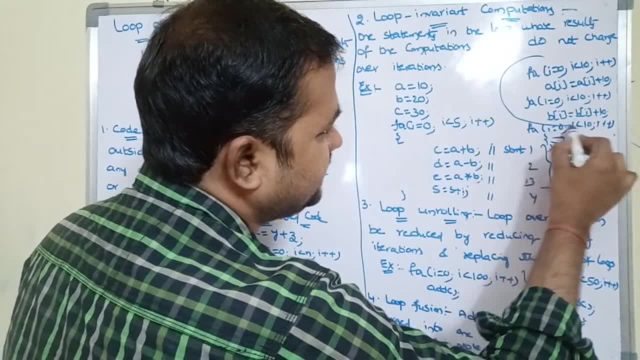 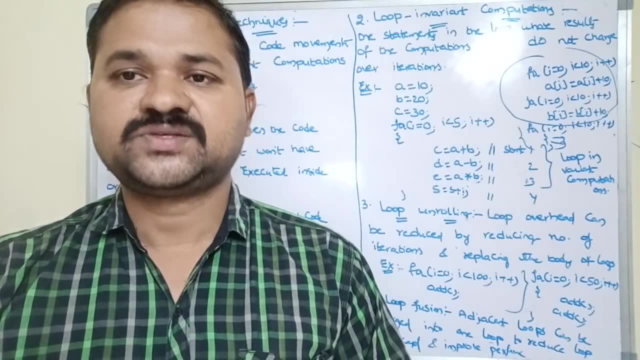 equal to B of i plus 10.. So we can eliminate these two for loops with the help of this for loop. So instead of writing two for loops, we can write only one for loop. So this is about loop optimization. 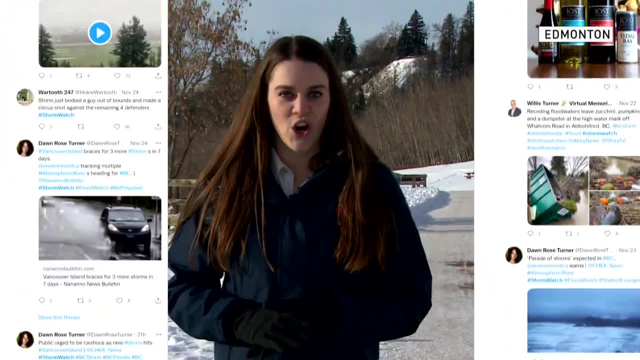 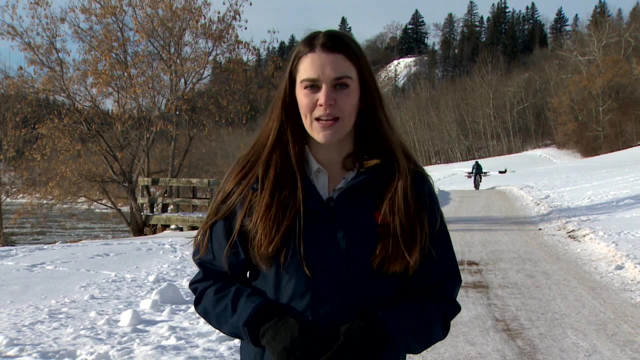 When a big storm hits, your social media feed is flooded with weather jargon- Low pressure system, atmospheric river, polar vortex- But sometimes even the most basic terms can be misleading. I'm talking about weather and climate. They're often used interchangeably.